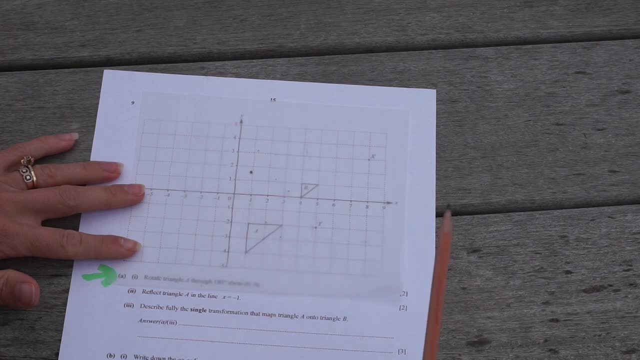 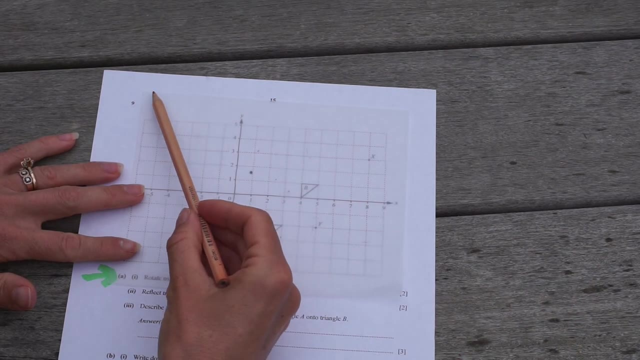 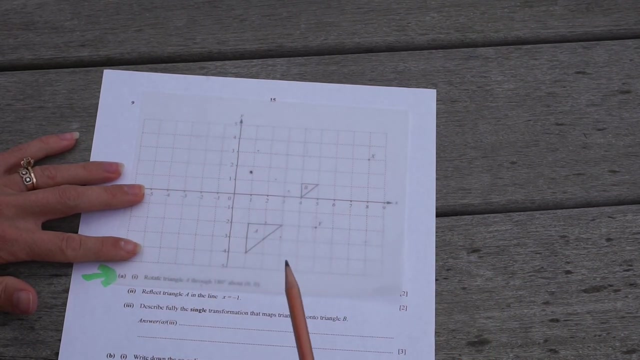 also the centre of your rotation And when you line up the paper, place it correctly. So when I say correctly, make sure the edges are aligned of your paper, are parallel to the x-axis and the y-axis, it will just make it a. 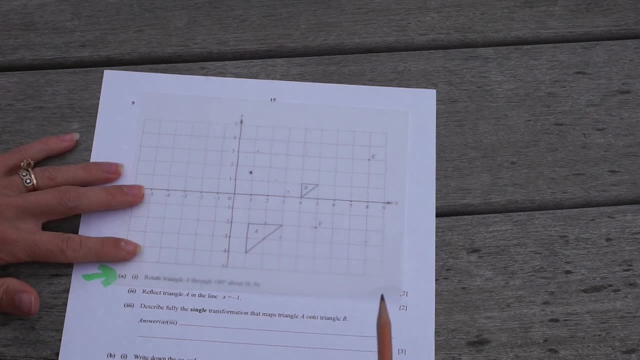 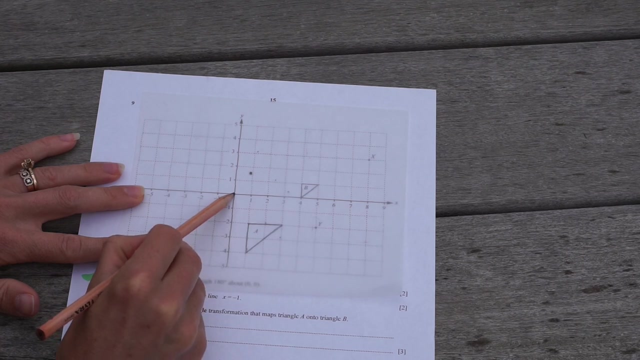 lot easier to count the number of degrees when you do the rotations. so next traced triangle a, okay, so there's triangle a, and then you need to place your pencil tip on the center of the rotation, in this case, zero, zero. now it says 180 degrees. that's half a turn. okay, half a turn in a full circle, and it. 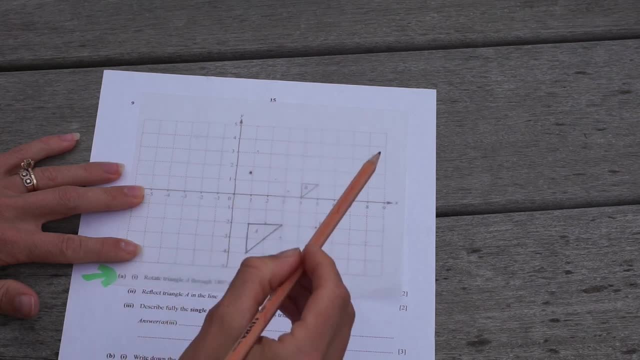 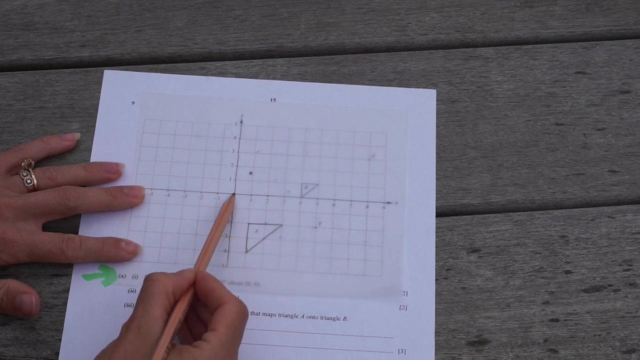 doesn't matter which way you turn, whether you're turning clockwise or anti-clockwise, it will give you exactly the same answer, but that's only if it's 180 degrees. that's the only exception when you don't need to state clockwise or anti-clockwise. so I'm going to turn my tracing paper 90 degrees to start. 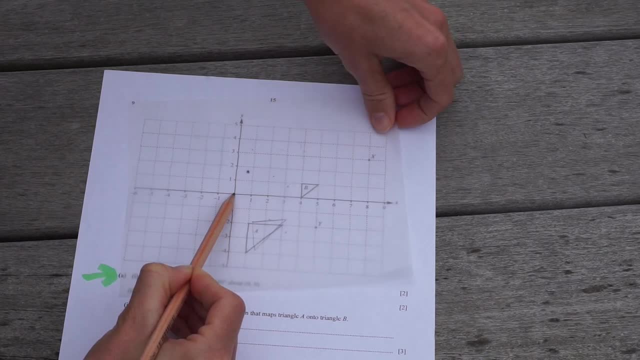 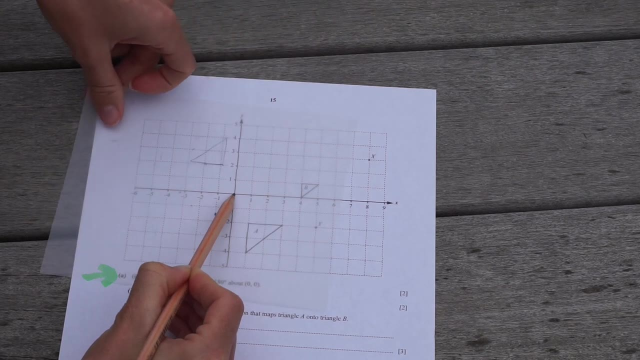 with. so a quarter of a turn, anti-clockwise. okay. so there's 90 degrees. then another 90 degrees takes me to here. so that is a turn of 180 degrees. so there's the new shape. okay, you have to draw triangle a in its new position up here. so just mark those points. 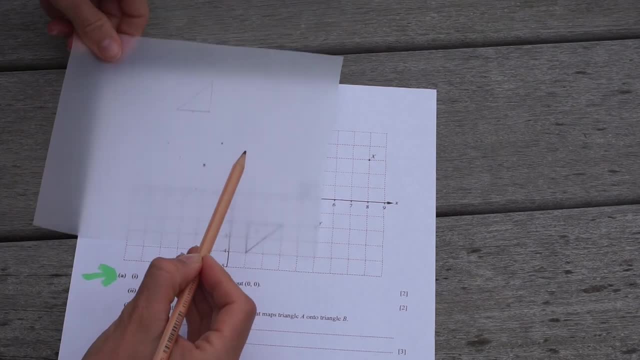 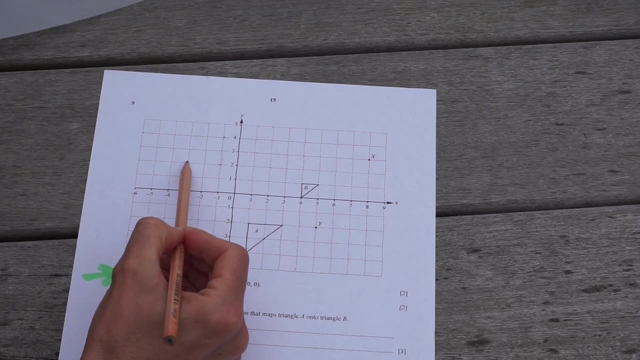 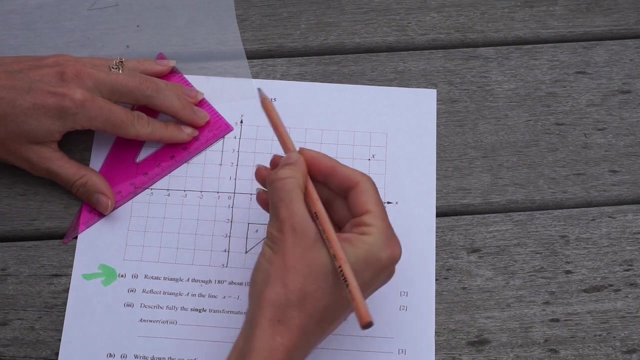 carefully. this point is at minus 12, this one is at minus one, four, all, and the last point minus one, four and the last point minus five, and it gets marked point is at minus three, two. okay, so once you've marked those in place, you can join them up. okay, so we've done the rotation, that's it. so when you're doing 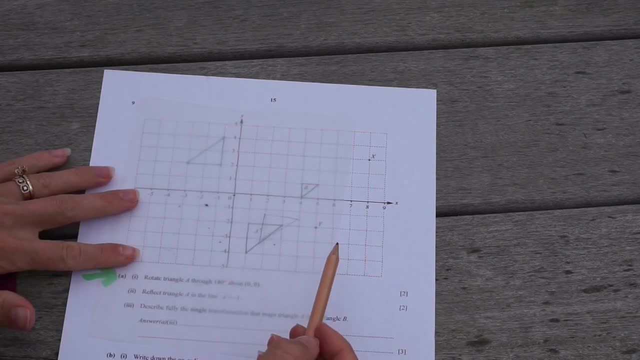 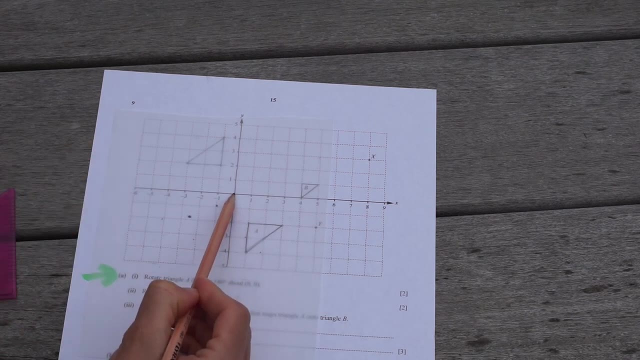 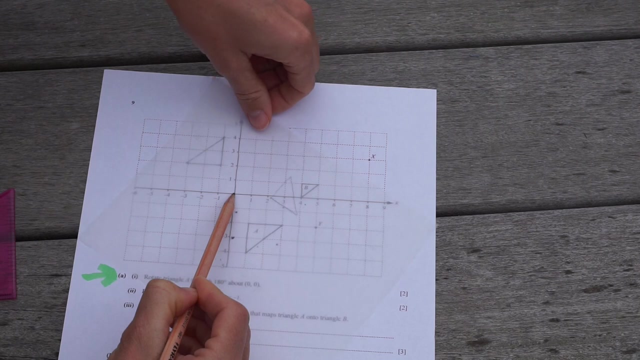 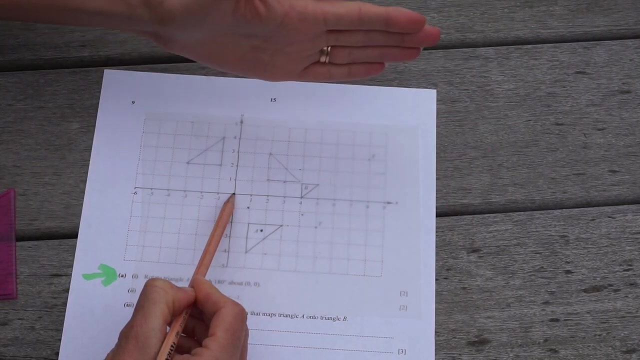 the rotation. if you're not sure about the number of degrees, it's quite handy to look at the edges of the tracing paper. notice how to start with. this edge here is vertical. when I've turned 90 degrees, that edge is now horizontal. so whenever the edge changes from vertical to horizontal or horizontal to vertical, 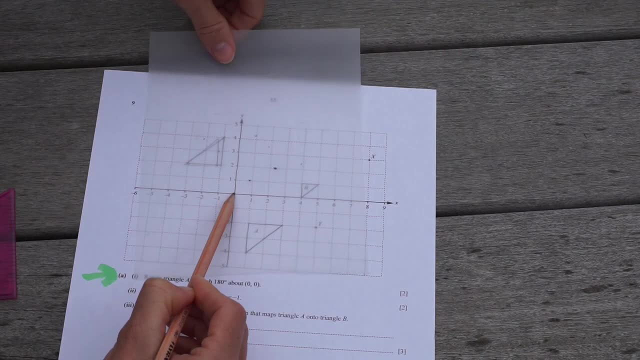 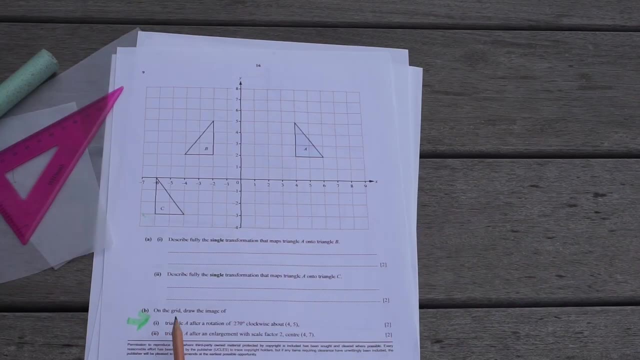 that's a turn of 90 degrees. okay, so that's just a little tip to help you count when you're doing the rotation. okay, okay. so in the next question it says on the grid draw the image of triangle a after a rotation of two 270 degrees clockwise, about 4.5.. 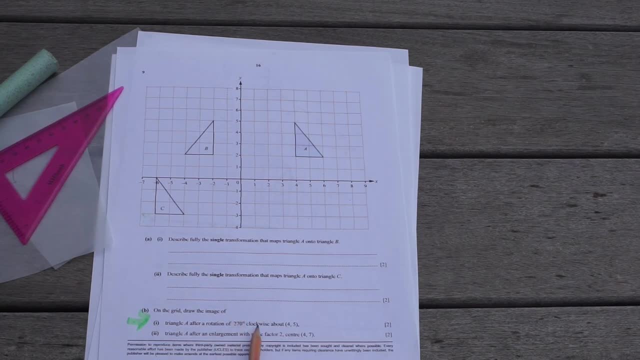 Okay, so 270 degrees clockwise is three quarters of a turn clockwise. So the same way as the clock. Okay, It's the same thing as turning 90 degrees anticlockwise. Okay, It doesn't matter which way you choose. Okay, you'll end up with the same thing. 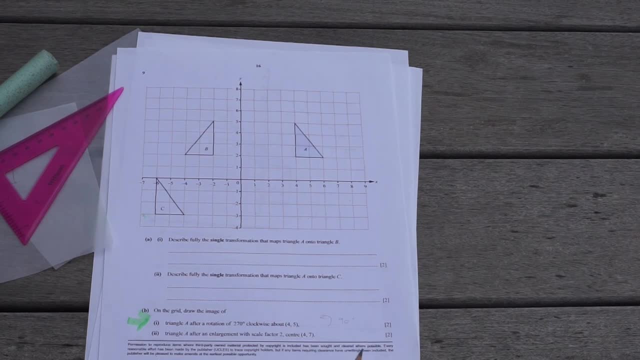 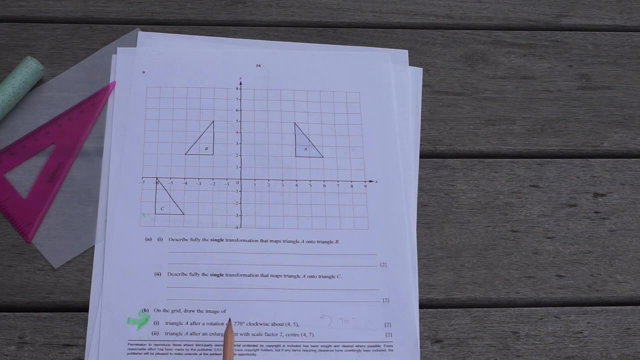 I'm going to do it this way because I think it's a little bit quicker and easier. So take your tracing paper and again trace the object triangle A, And when you do that, make sure that your tracing paper also lies over the point 4, 5.. 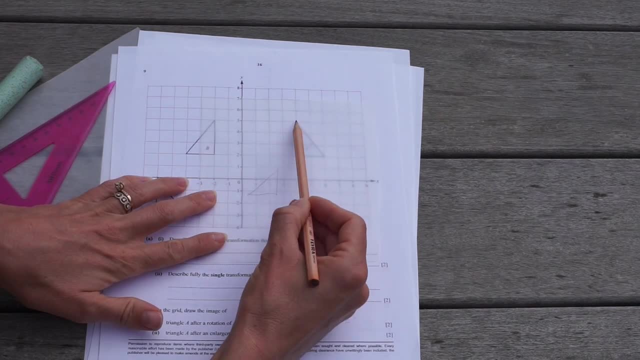 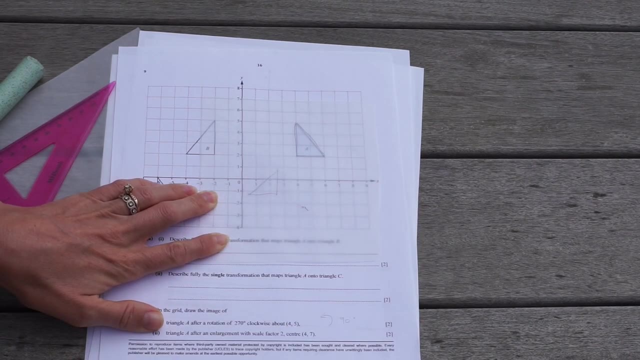 Okay, so that's easy because 4, 5 is on the triangle here. Okay, so trace the shape. So next you need to place your pencil tip on the centre of the rotation 4, 5.. So here. 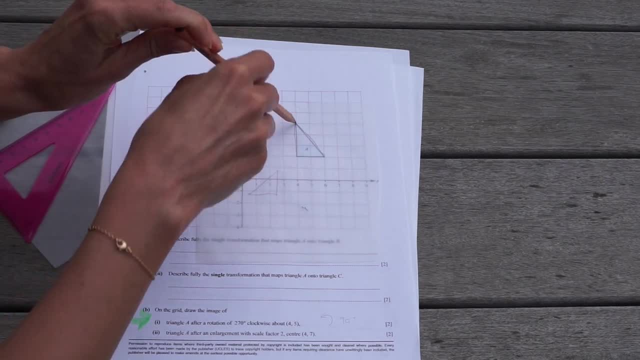 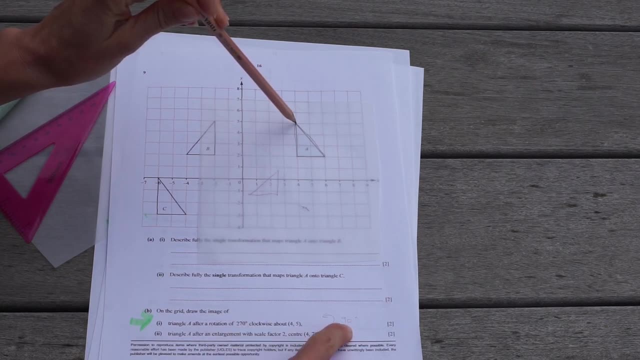 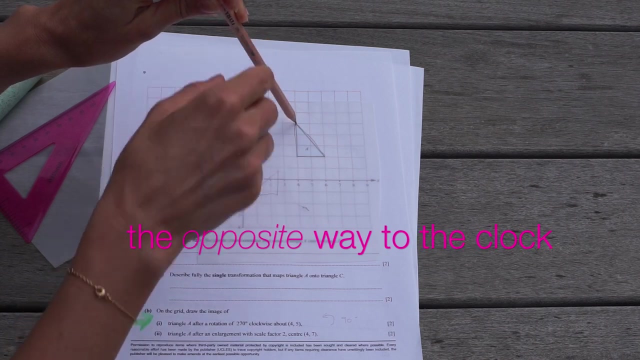 And then you need to turn your paper 90 degrees anticlockwise, or 270 degrees clockwise, if you prefer. Okay. so 90 degrees anticlockwise is one quarter of a turn. Okay, the same way as the clock. So notice how the tracing paper is like this at the moment. 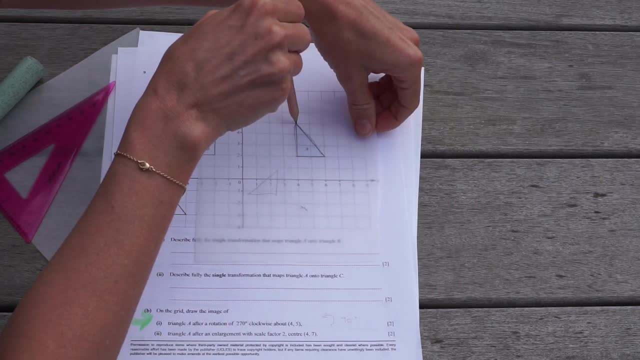 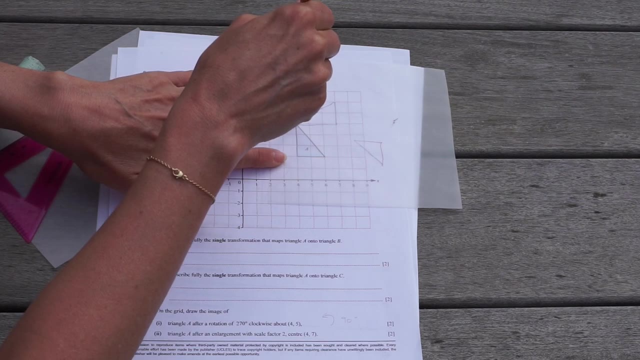 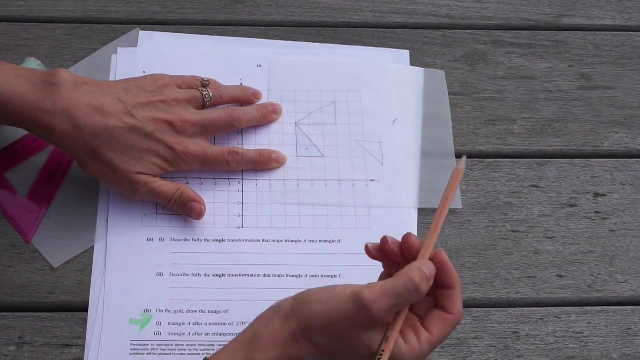 Okay, on the right hand side, That vertical edge needs to become horizontal, Okay, Okay. So there we've done a 90 degree turn, a quarter of a circle. Okay, there's the new shape here. So again, look very carefully at where your shape is when you take the tracing paper away. 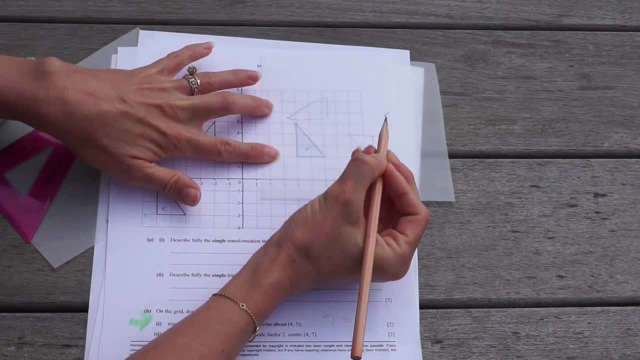 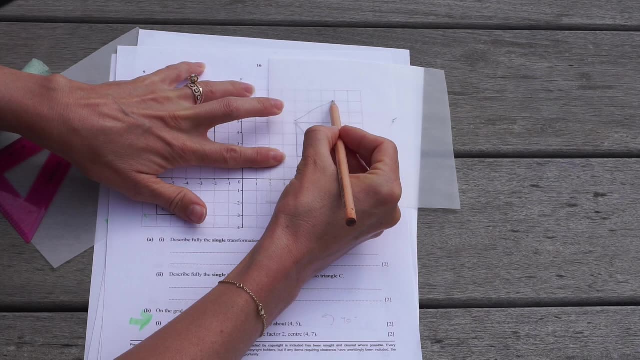 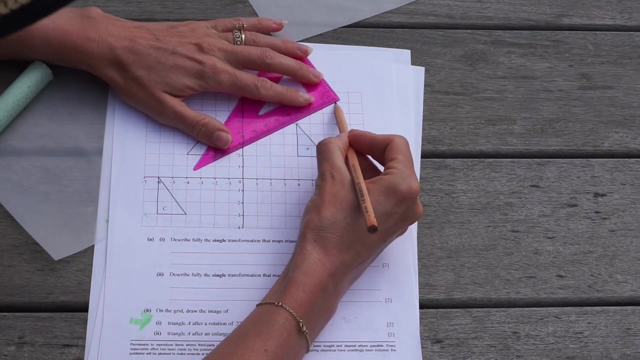 So this point is on the centre 4, 5.. This point here on the triangle is at 7, 5.. And the final point here is at 7, 7.. Okay, so once you've got all your points in their correct place, you can join them up. 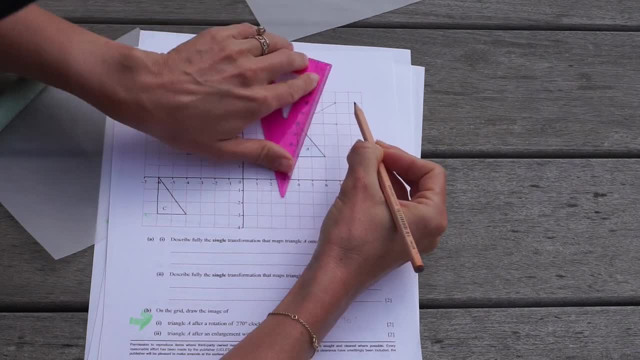 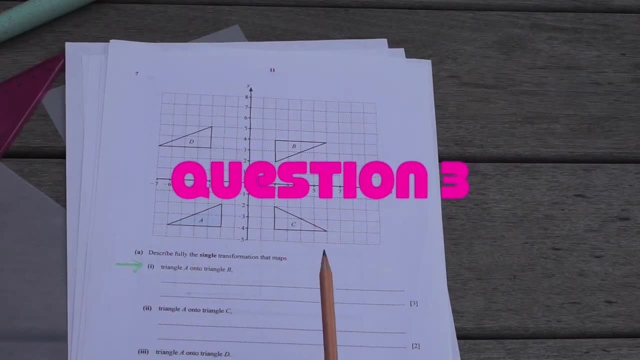 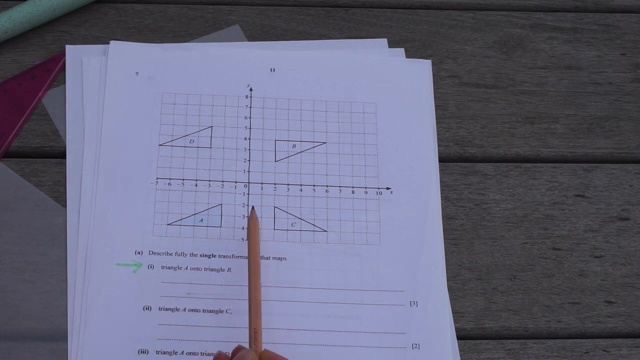 And there's the rotation. Okay, so that's the image of A after the turn. Okay, so in this question it says: Describe fully the single transformation that maps triangle A onto triangle B. So here's triangle A, Here's triangle B. 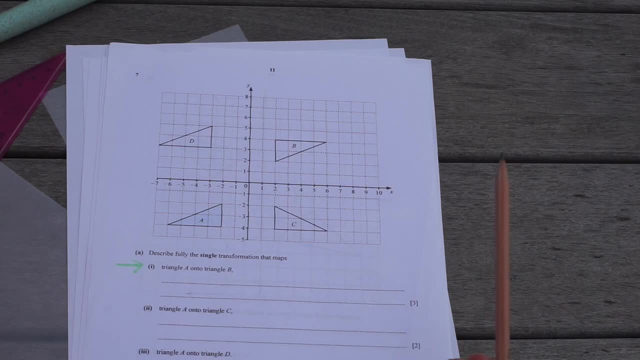 We can see the shape has turned And it's the same size, So it's a rotation. So you would write down the word rotation, Okay, Next you take your tracing paper and you need to try and find the centre of the rotation. 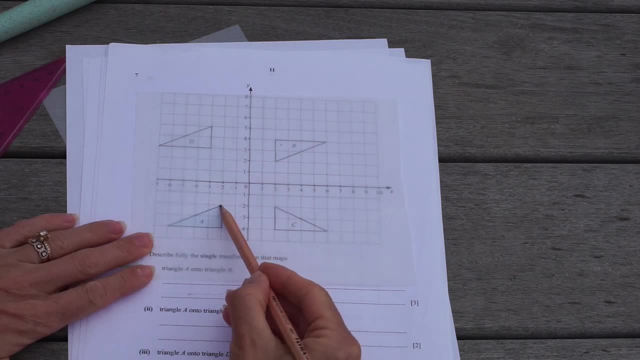 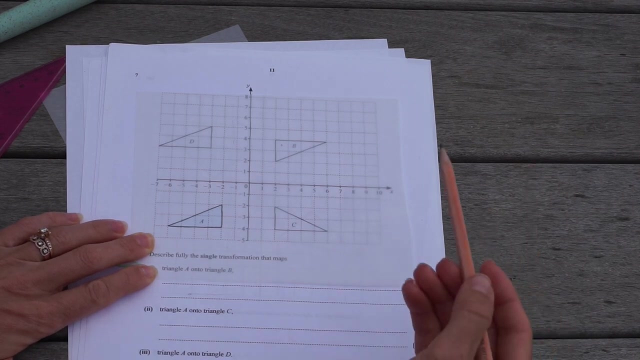 Okay, so take your tracing paper and trace triangle A And then you would just test a point to see when you turn around that point does it end up on triangle B. So I'm just going to try this point here. 1, 1.. 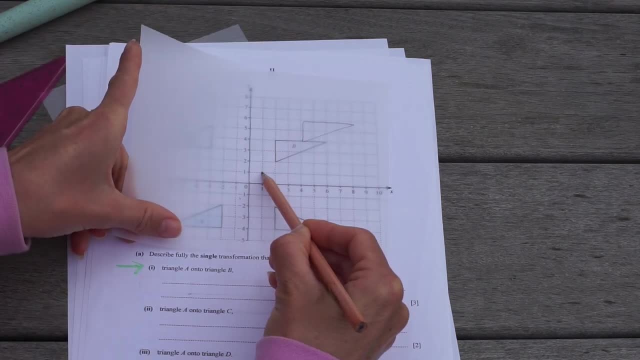 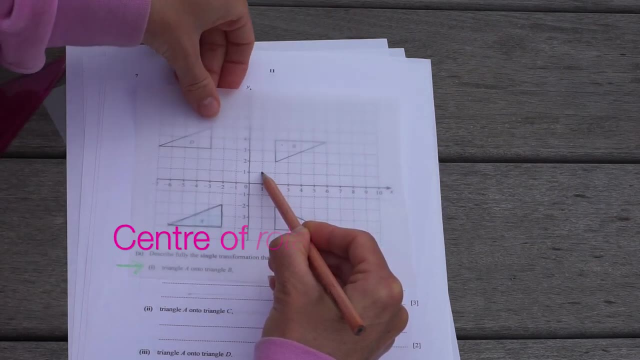 And if I turn the paper around, I'm going to see if it's on triangle B. And if I turn the paper around, can you see it doesn't line up exactly on triangle B, So I haven't quite chosen the correct centre of the enlargement, but I'm close. 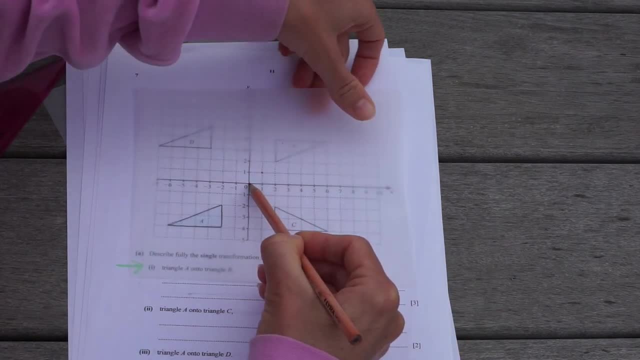 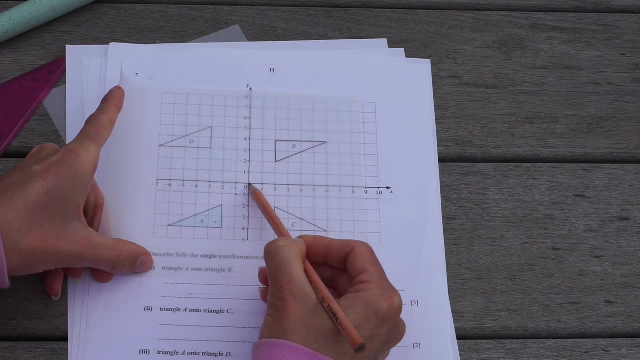 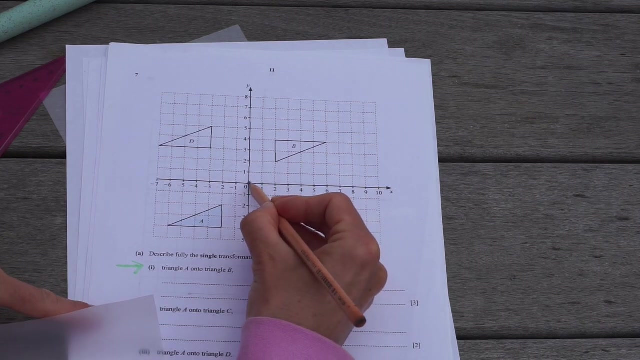 Next I'm going to try the origin. Okay, so 0,, 0. And this time when I turn the tracing paper, it ends up on triangle B. So I found the centre of the rotation. Okay, A good little trick when you're looking for the centre of the rotation is that this centre point is always. 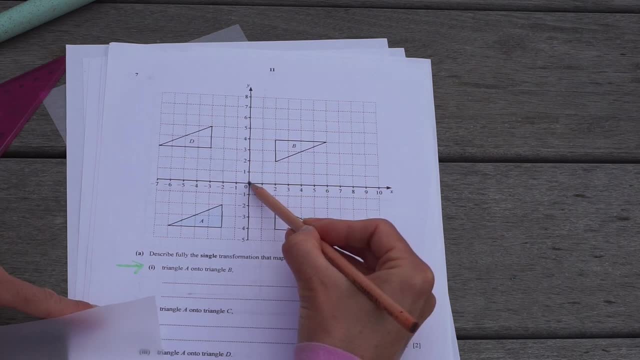 always the same distance to the corresponding points in triangle A as it is to triangle B. So can you see that this point here on triangle A corresponds to this one on triangle B. This is two squares across to get to the centre, and likewise with this point. 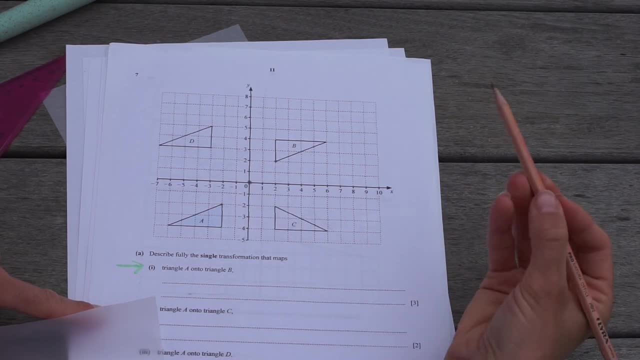 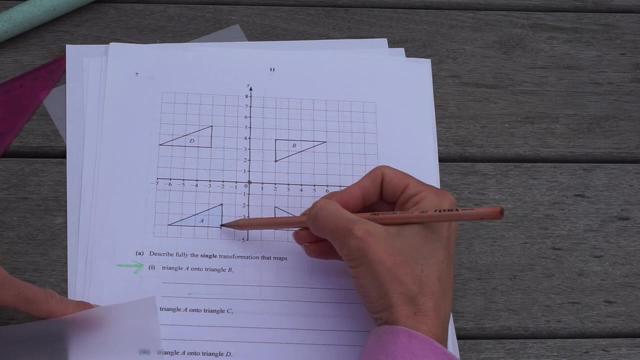 Okay, they're the same distance to that centre point. Now, if you take another pair of points, for example these two, you'll find that they are also the same distance To the centre of the rotation. So that's a good little trick to find the centre of the rotation a bit more quickly. 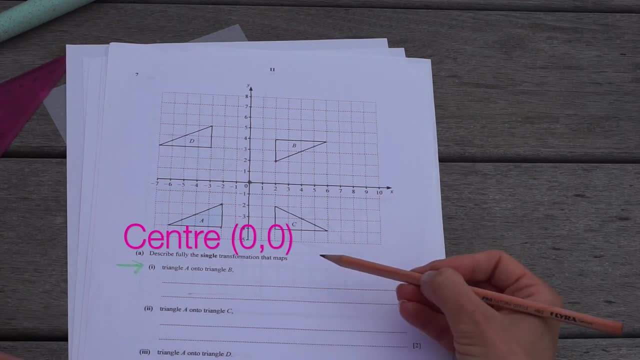 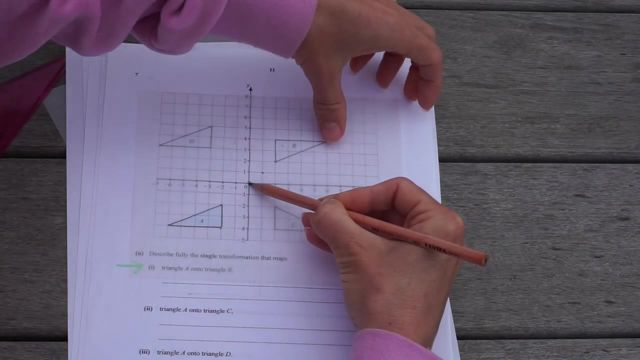 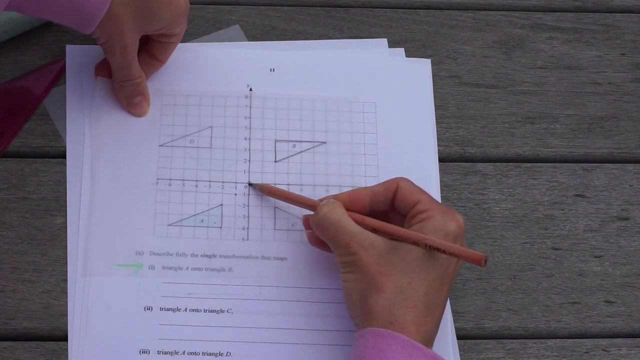 So the next part of your answer you would write down is centre 0, 0.. Okay, the coordinates Now. hopefully you saw when I turned to get from triangle A to triangle B it was two quarter turns, so half a turn, which is 180 degrees. 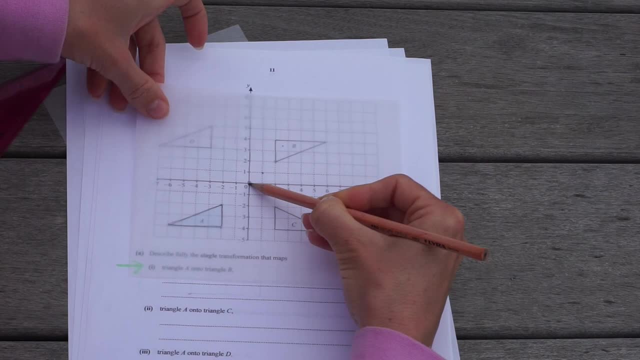 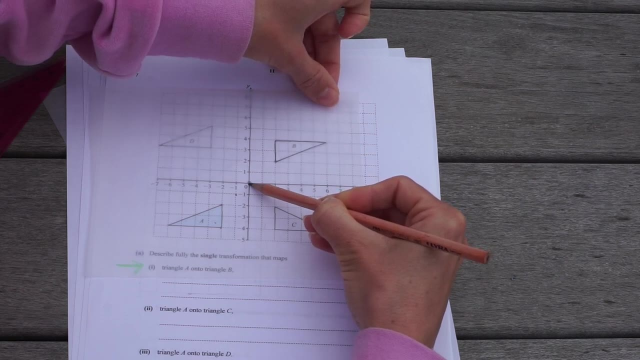 Okay, Okay. And just like I showed you at the beginning of the lesson, it doesn't matter which way you turn 180 degrees- clockwise or anticlockwise, it will give you the same result. So you don't need to state clockwise or anticlockwise in this question. 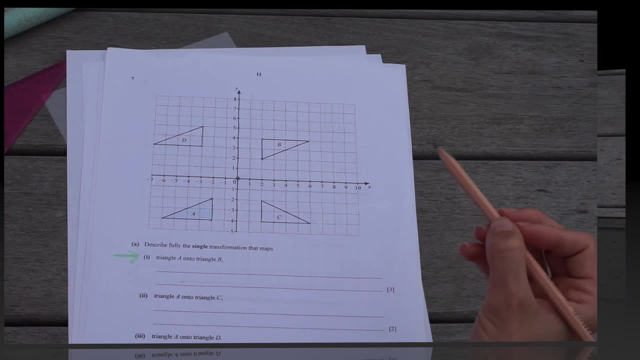 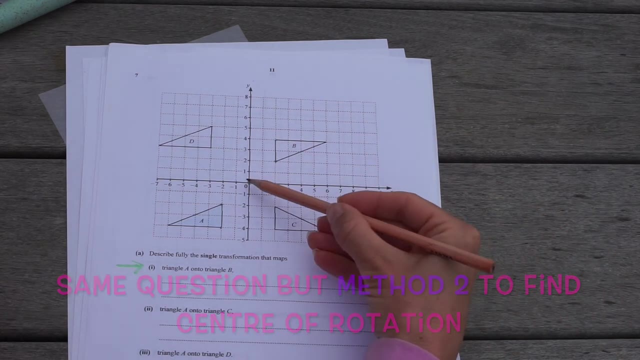 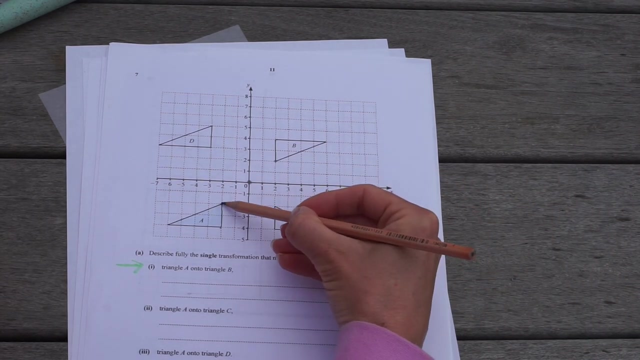 You would just write down 180 degrees. Okay, so before we move on to the next question, I am going to just show you the other method to find the centre of the rotation more exactly. So take two corresponding points, So for example this point here on B and this point on A, and join those up. 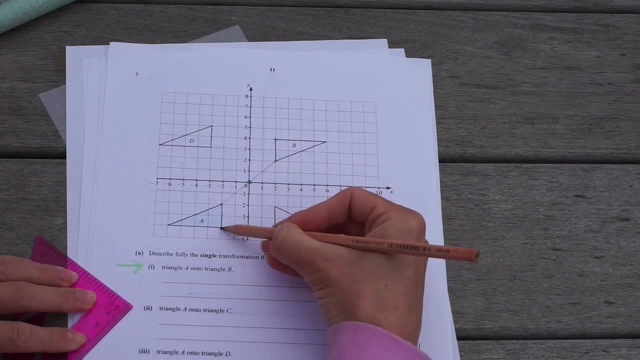 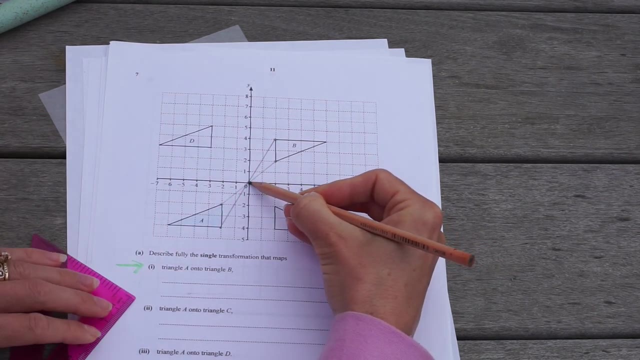 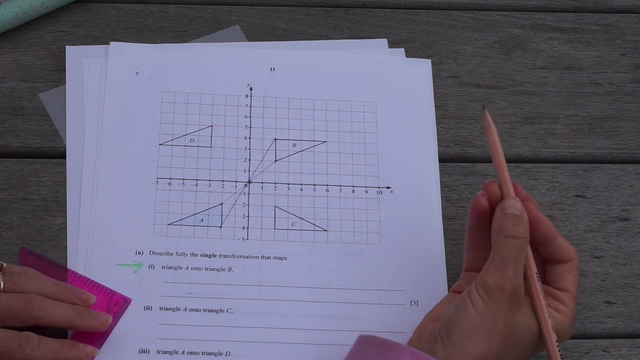 And then take another pair of corresponding points on the two triangles, So those two, for example, and join them up. And it's just a coincidence that they cross over the centre. Okay, we're not quite finished. Then what you would do is find the perpendicular bisectors of those two lines. 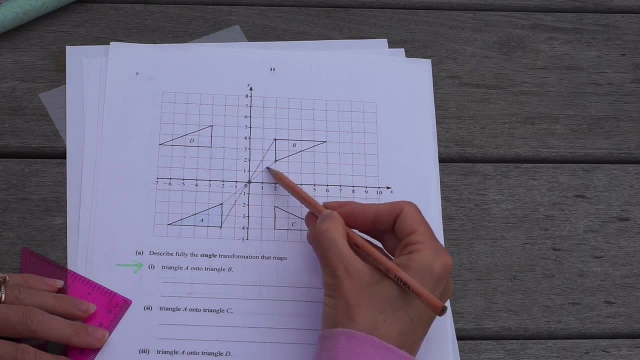 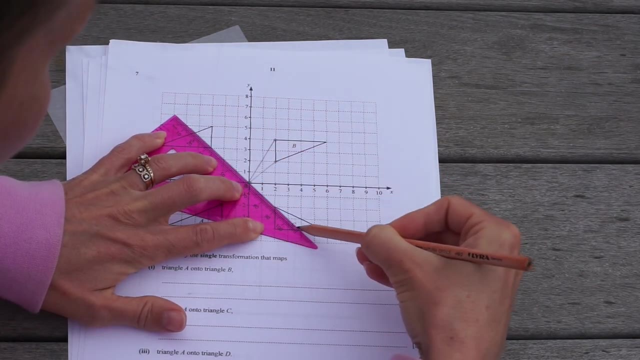 So let's look at the first line. this one here Halfway along the line is here And perpendicular to that line is at 90 degrees. So you would draw that line there. Then you would take the other line that you drew connecting those two points on the two different triangles. 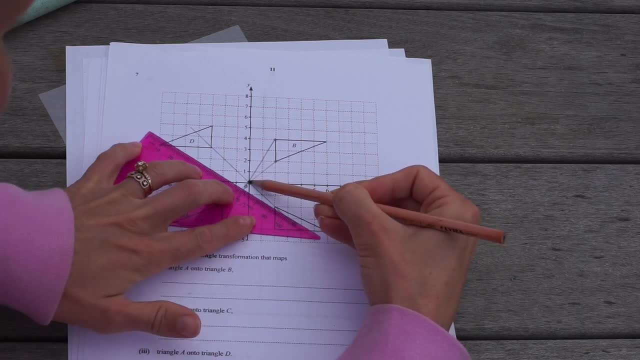 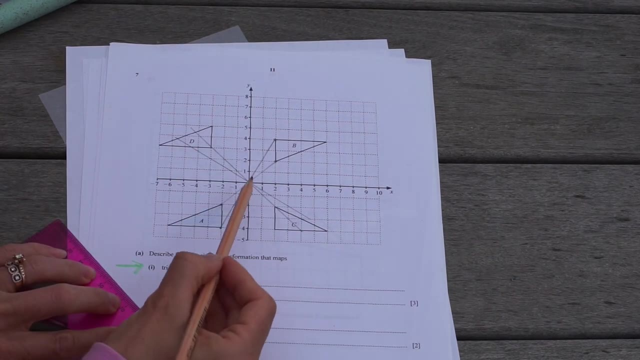 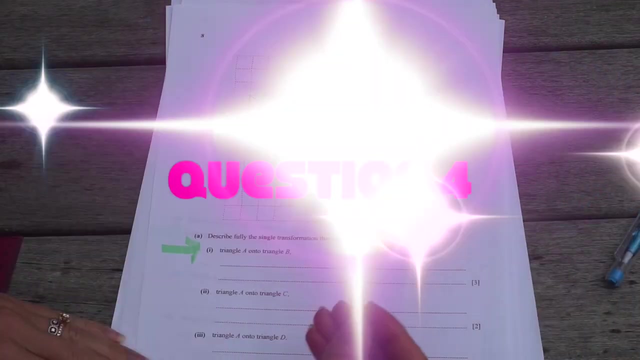 Halfway along the line is here And perpendicular to the line at 90 degrees is there. So those two lines that I just drew cross at the origin. So that is the centre, That is the centre of the rotation. So in this question it says: 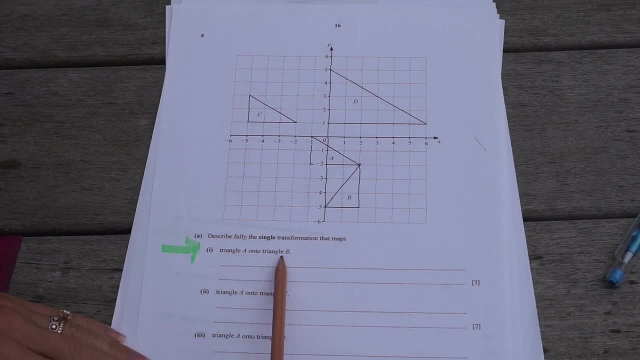 Describe fully the single transformation that maps triangle A onto triangle B. So here's triangle A and here's triangle B. Well, it's a rotation. Okay, we can see the shape has turned Okay in this transformation And the shapes they're the same size. 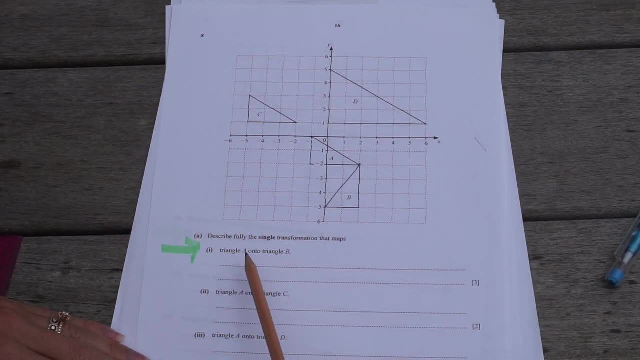 Okay, we say they're congruent. So the first thing you would write down is the word rotation. Next we need to try and find the centre of the rotation. So to start with, I'm just going to use a method, logic, to find the centre of the rotation. 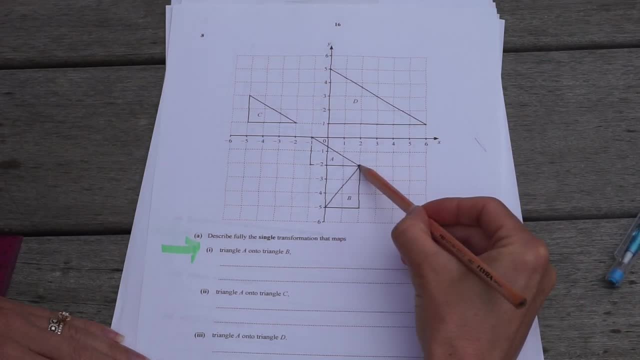 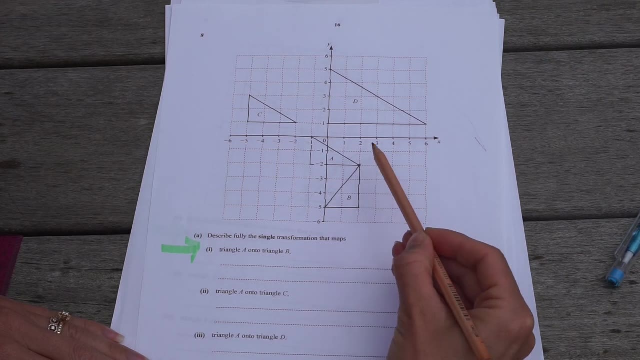 I can see that the centre of the rotation is here: 2 minus 2.. A little trick you can use just to help you find the centre of the rotation is that this centre point must be the same distance to all the different pairs of corresponding points in the two triangles. 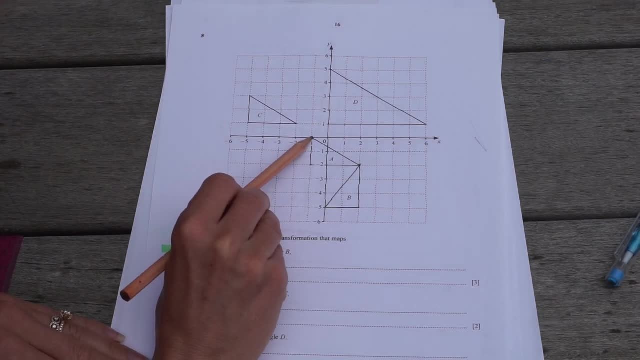 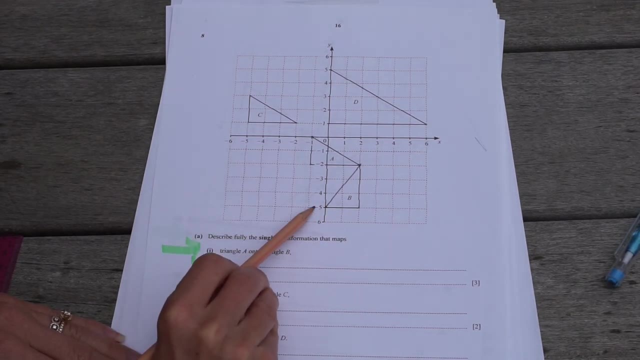 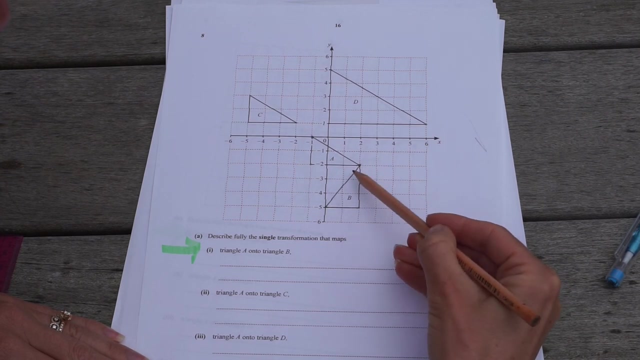 So, for example, this point of the triangle A Corresponds to this point on triangle B. Okay, so this point becomes the point here after the rotation, And these points are the same distance to the centre of the rotation. Likewise, if we choose a different pair of points, 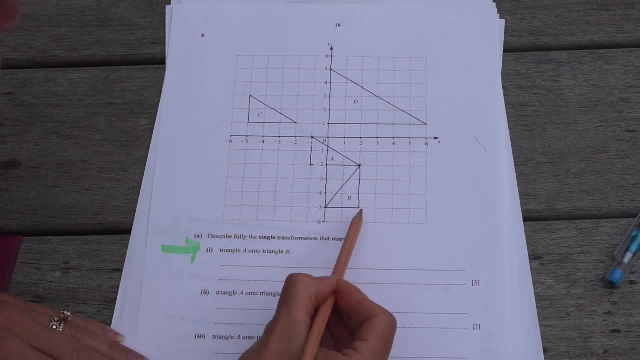 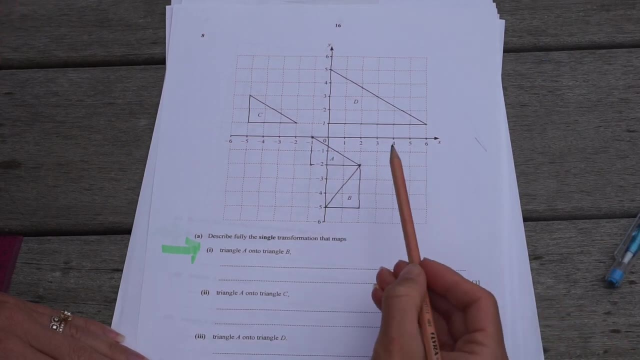 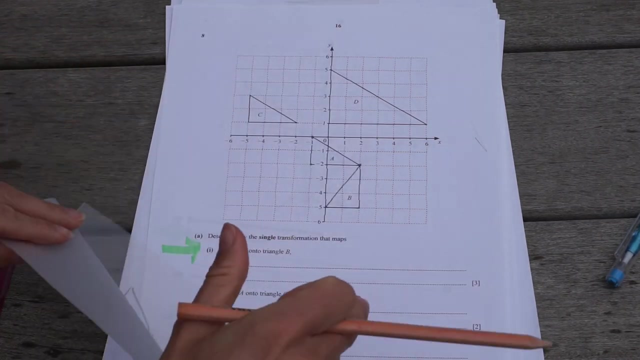 This point here and this point here. They correspond to each other. They're also the same distance to the centre of the rotation. Okay, so you would write down centre 2 minus 2.. And you can just check with your tracing paper to make sure you're correct. 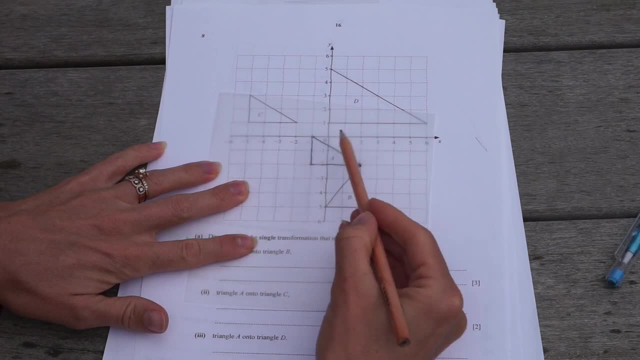 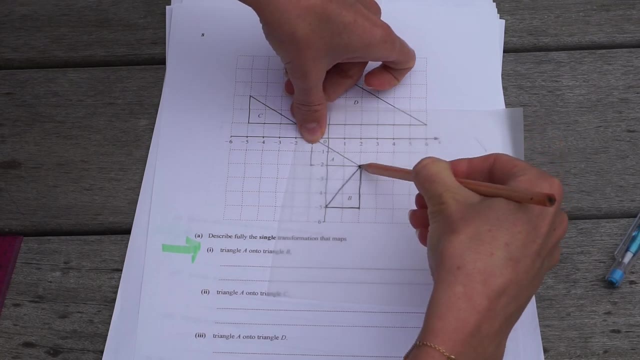 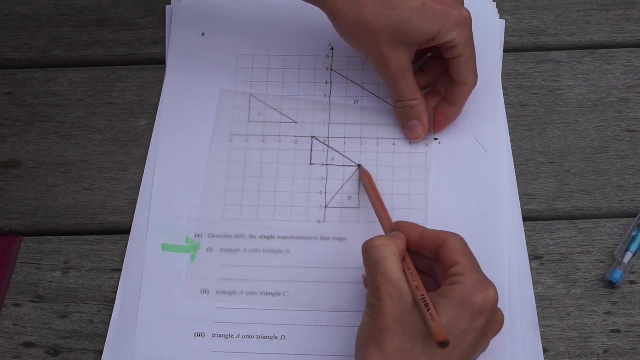 Okay, with your centre Trace, triangle A, Put your pencil tip on the centre, Turn And because it lines up exactly on triangle B, we know that the centre is correct. Okay, Hopefully you can see that to get from triangle A to triangle B, it's a rotation of 90 degrees, anticlockwise. 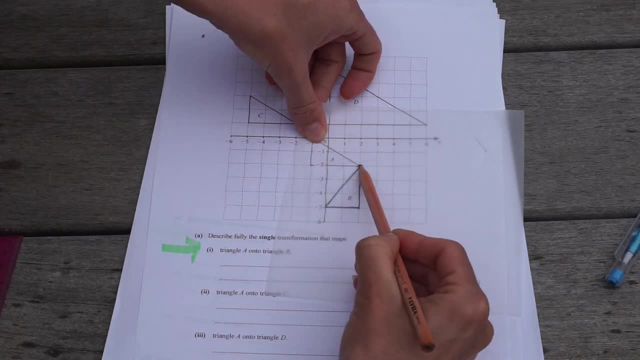 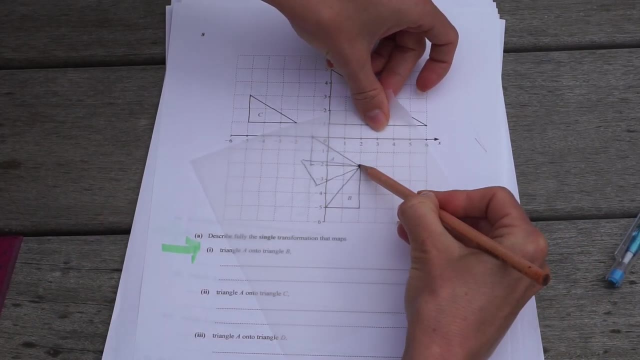 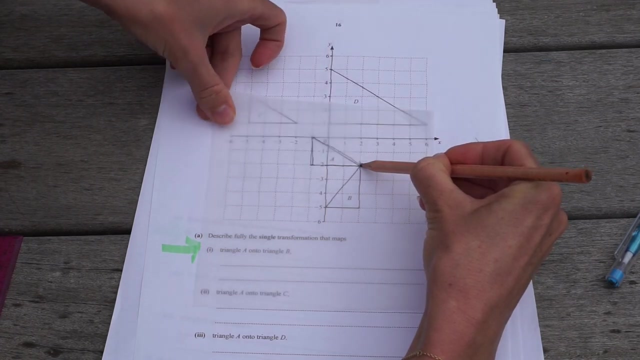 Because I'm turning against the clock. Okay, in that direction. You can see, to start with the tracing paper edge here is vertical And then after a quarter turn here it becomes horizontal. Okay, so it's 90 degrees. You could also say, to get full marks, 270 degrees clockwise. 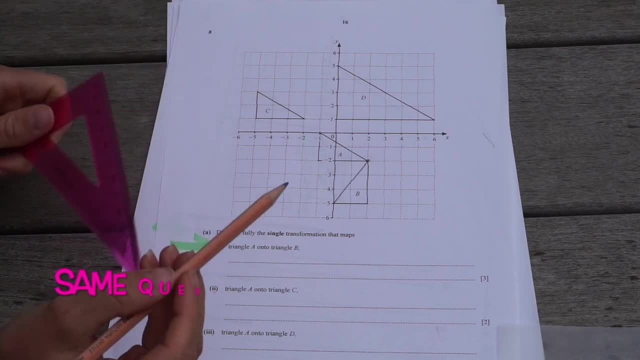 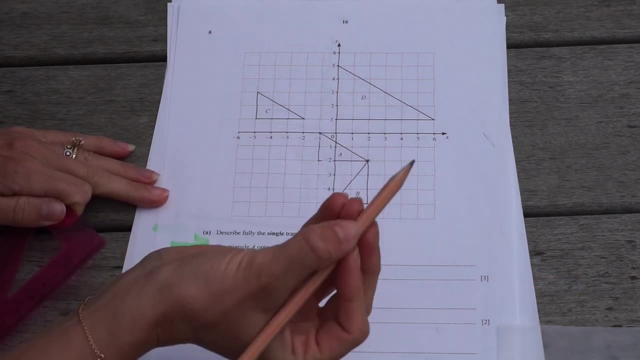 Okay, because that's the same thing. Take a ruler or a straight edge And join up the pairs of corresponding points On the two different shapes. So when I say corresponding points, I mean this point on triangle A, after the rotation ends up here. 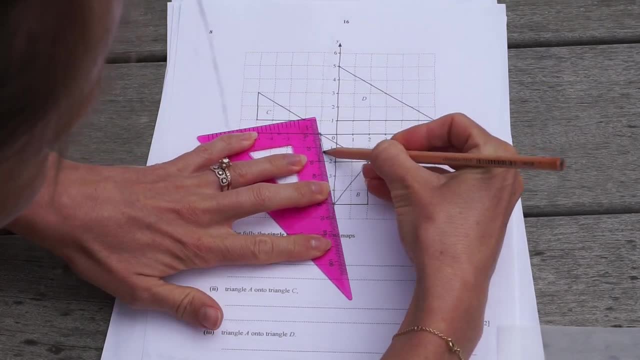 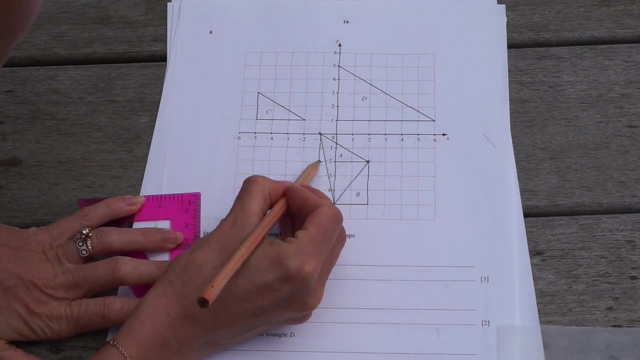 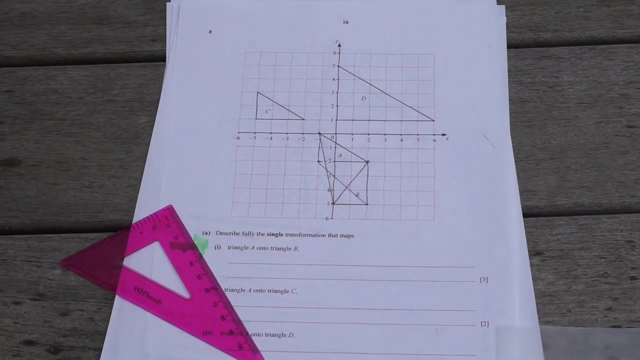 So you must join those two points up. Then you need to do the same thing with a different pair of points, So for example this point on triangle A, after the rotation ends up here. So then you can join those points up. Next you need to draw the perpendicular bisectors of those two lines. 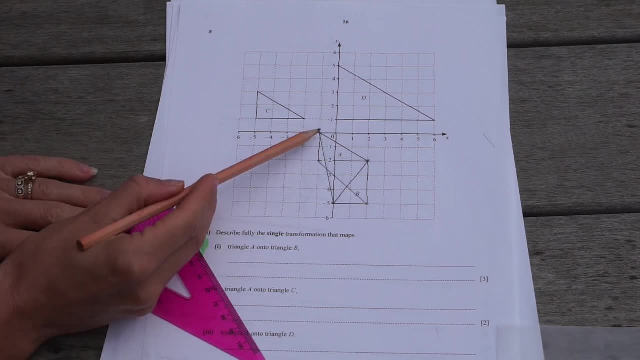 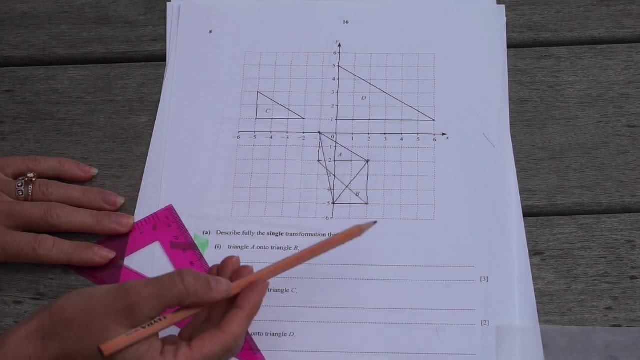 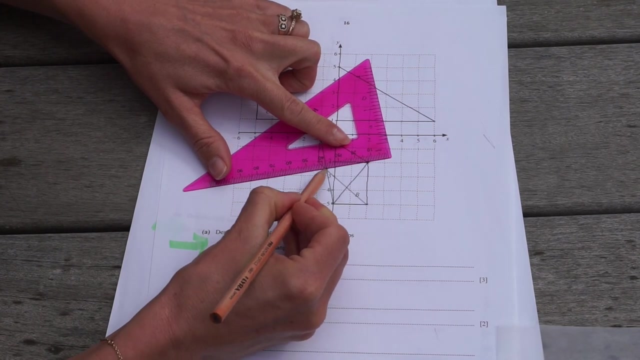 So the perpendicular bisector is just a line that's perpendicular, So at 90 degrees to this line, But halfway along this line. So halfway along this line is here, And if I draw a line that's at 90 degrees to that line across my grid, 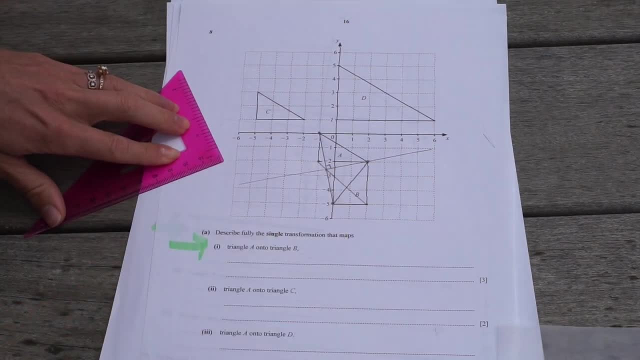 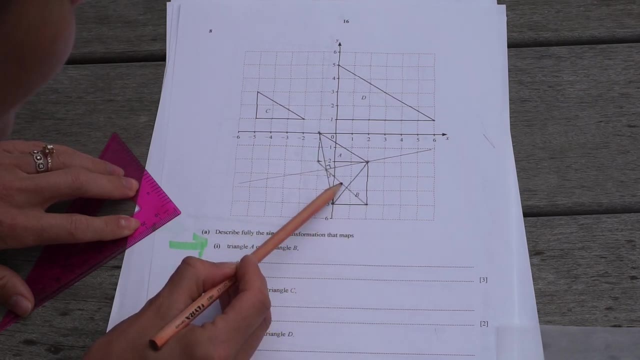 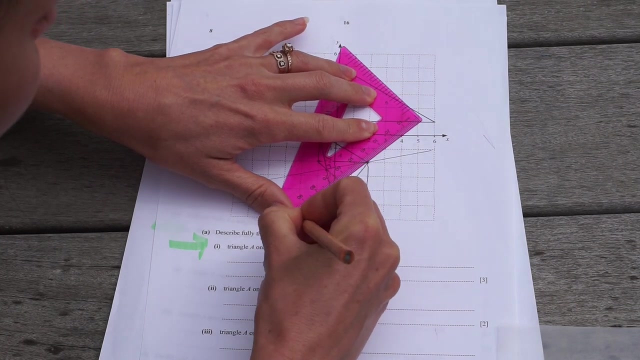 It would look like that: Okay, so that's at 90 degrees. Then you need to do the same thing with the other line that you drew, So halfway along the line is here, And then when you draw the perpendicular bisector, So a line at 90 degrees to that line across your grid. 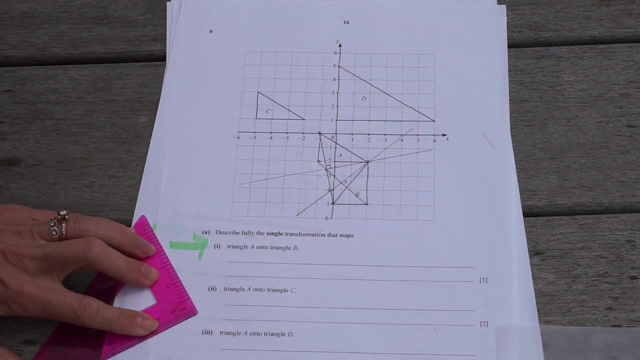 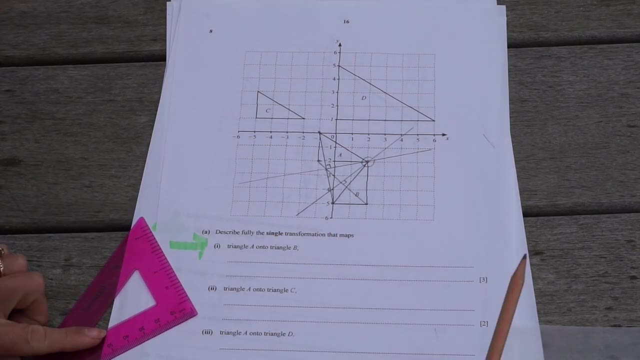 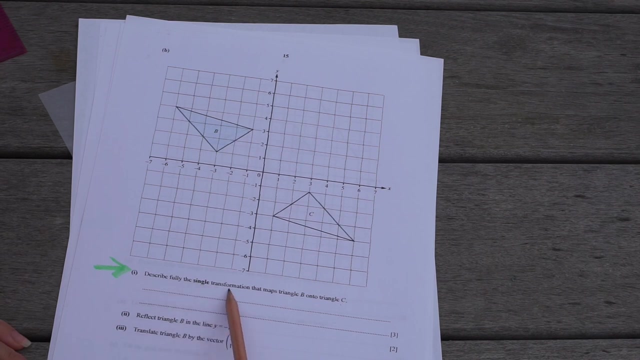 It would look like that Those two lines cross at the center of the rotation, So that is a more accurate method of how to find the center of a rotation. Okay, in this question it says: Describe fully the single transformation that maps triangle B onto triangle C. 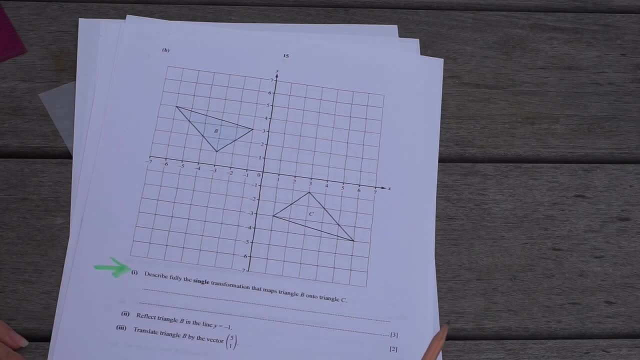 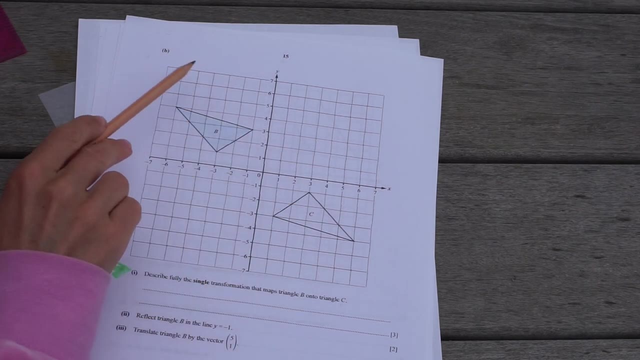 So here's B and here's C, So we can see it's a rotation. Okay, it's not a reflection. Okay, because the points haven't been reflected onto each other. It's turned. Okay, so you would write down the word rotation for the first part. 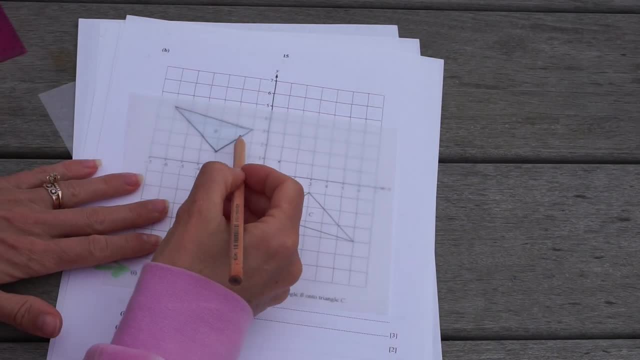 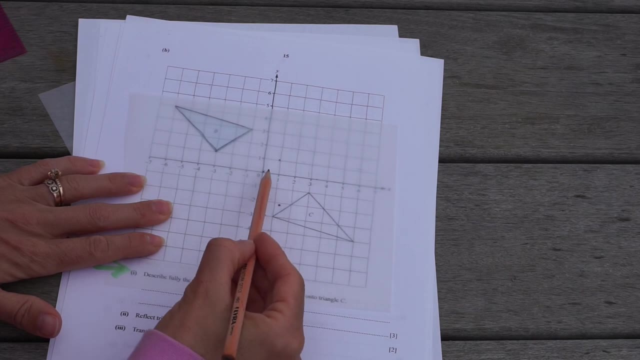 Next you would trace your triangle B, Okay, and then you have to try and find the center of the rotation. Now it's often Often the origin. So I'm going to look at the origin here And I can see that the points do look as if they are exactly the same distance from the center. 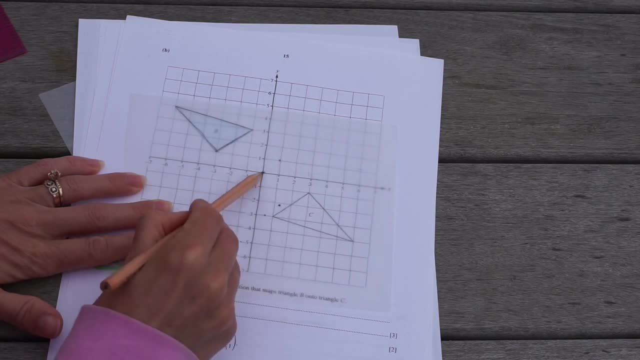 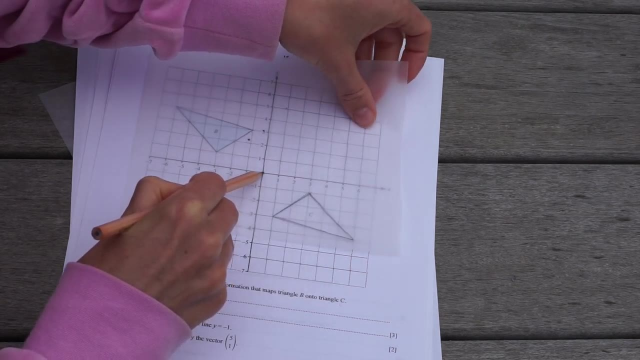 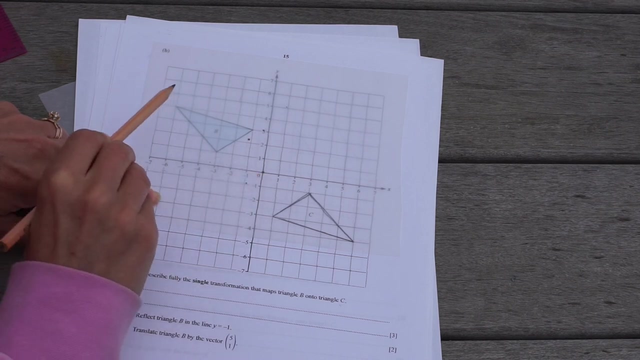 Okay when I compare the different pairs. So let's see: Okay, there's 90 degrees, Another 90 degrees, And indeed it is the center of the rotation. So you would write down center 00.. And because I did half a turn, 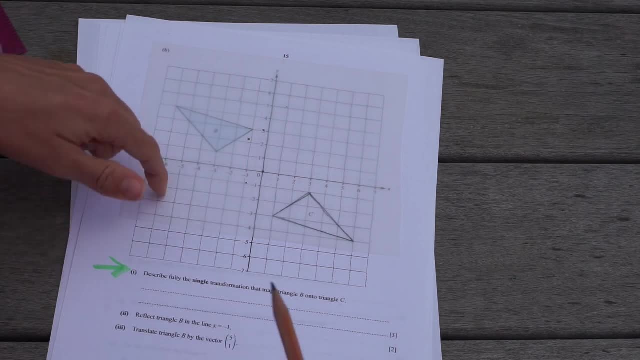 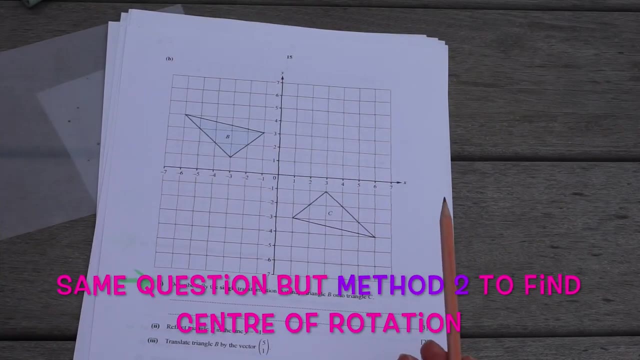 It's 180 degrees And remember, you don't need to write whether it's clockwise or anticlockwise whenever it's 180 degrees. So I'm just going to show you the method of how to find the center of the rotation accurately one more time. 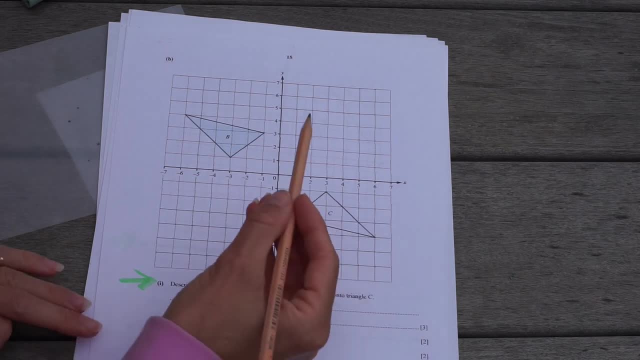 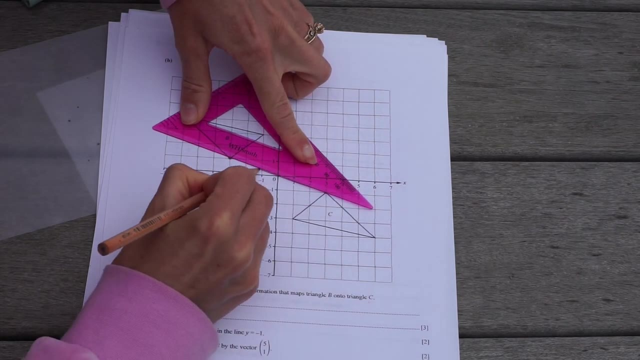 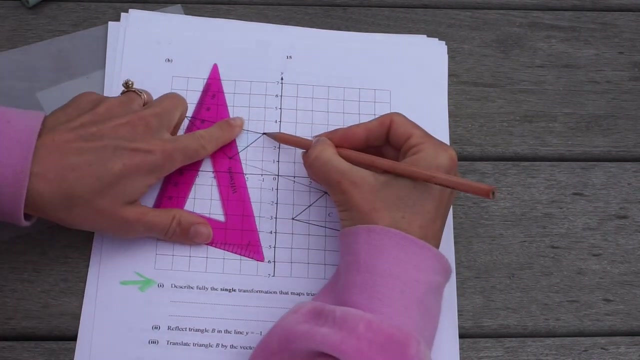 So you would choose the corresponding points on the two different triangles, So this point corresponds to this one, And you join them up with a ruler And then find another pair of corresponding points. So, for example, this one and this one, Join them up. 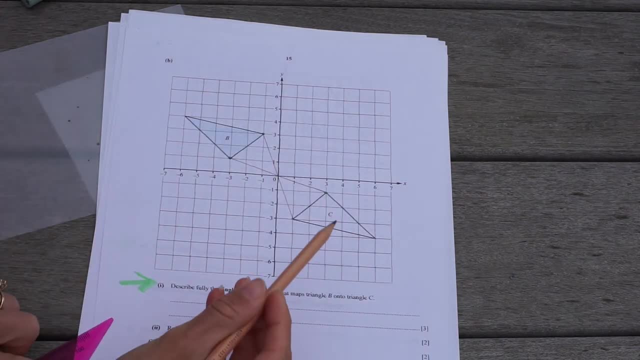 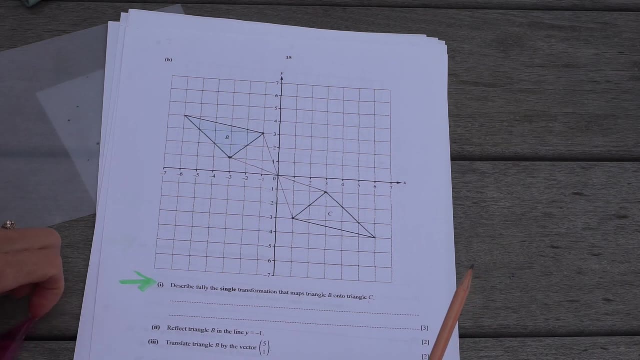 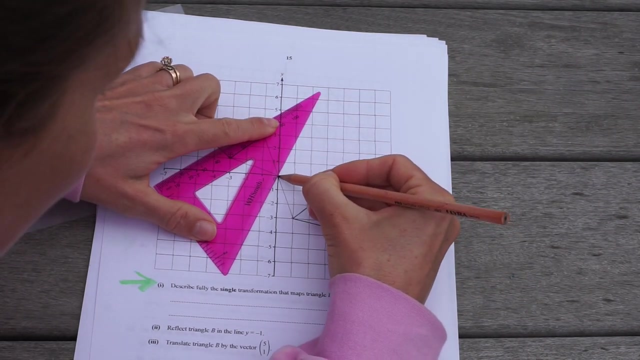 Now remember, it's just a coincidence that these lines cross on the center of the enlargement. It's not always the case at this stage. Then you would find the perpendicular bisectors of those lines. So halfway along, this line is here And the line that's perpendicular is at 90 degrees. 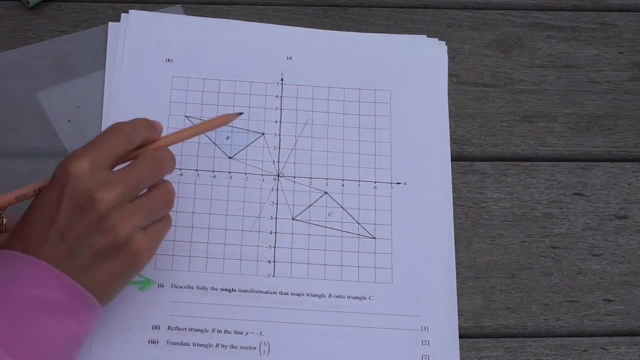 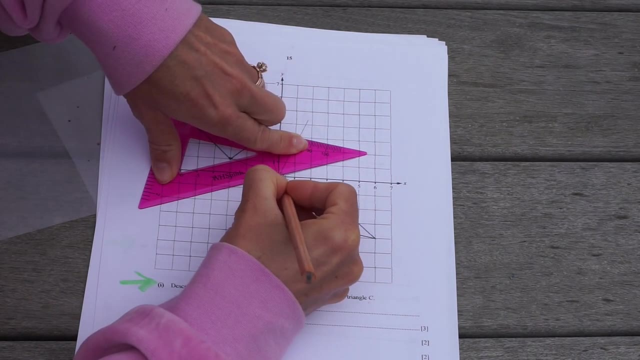 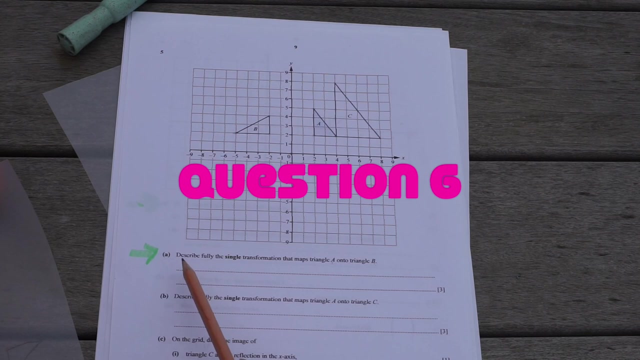 So like this: And then halfway along this line is here, And at 90 degrees we do this, And those lines cross at the center of the enlargement, The origin 00.. So in the last question it says: describe fully the single transformation that maps triangle A onto triangle B. 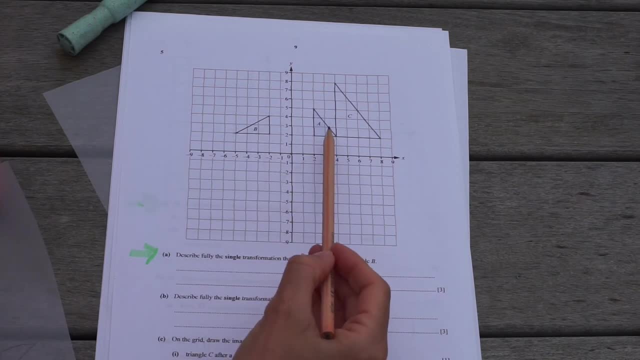 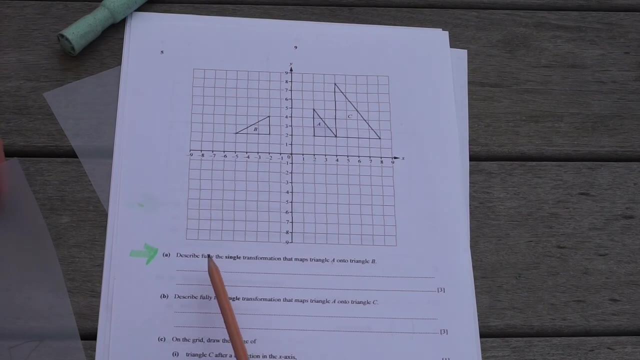 So here's triangle A and here's triangle B. We can see it's a rotation, because the shape has turned And the shapes are the same size. So the first thing you would write down in your answer is the word rotation. Now let's try and find the center of the rotation. 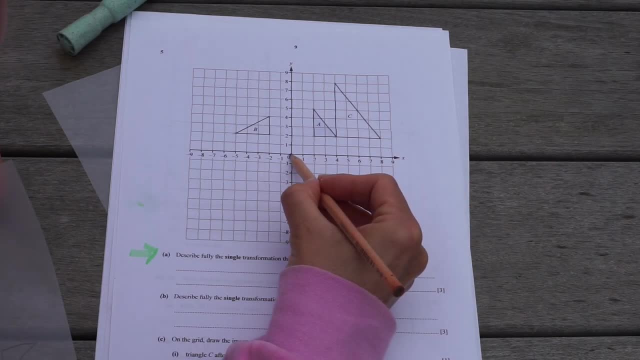 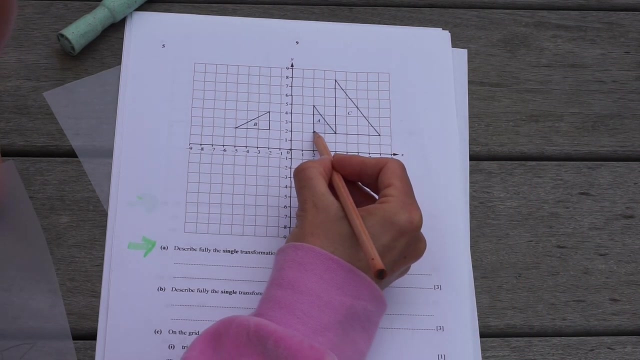 Well, if we look at the origin, we can see that this center point is the same distance to all the pairs of corresponding points in the two different shapes. So when I say corresponding, I mean this bottom left hand corner of triangle A. after the rotation is then here: 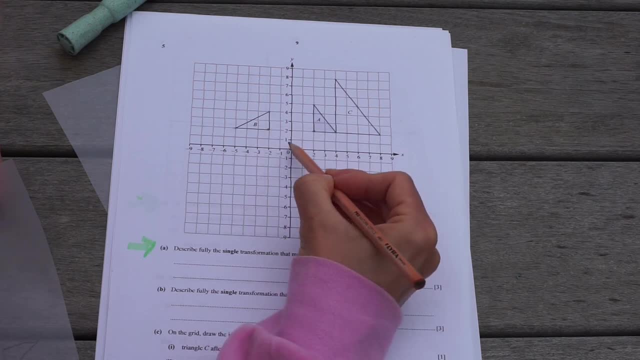 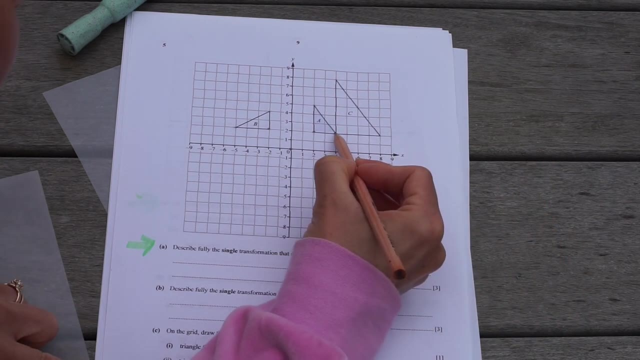 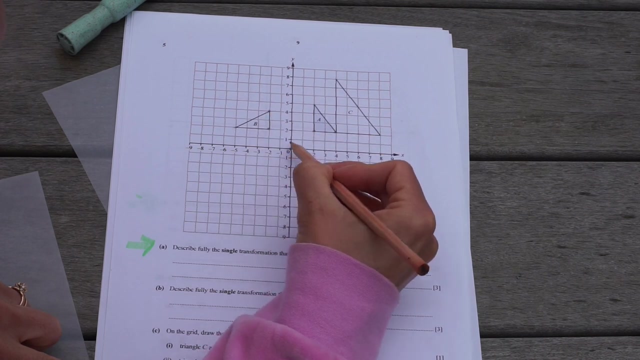 Okay, Those corresponding points are exactly the same distance To the origin. Then if we take a different pair, For example the bottom right hand corner of A after the rotation, it changes to this position: These two points are also the same distance to the origin. 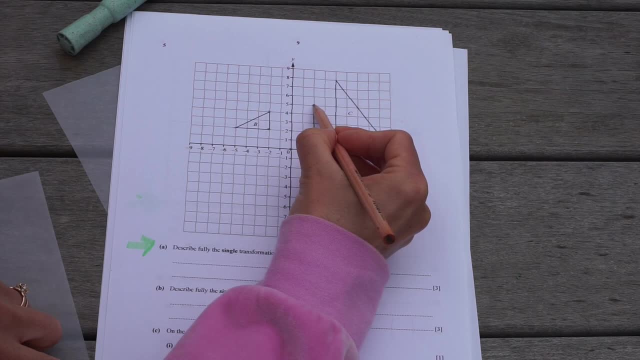 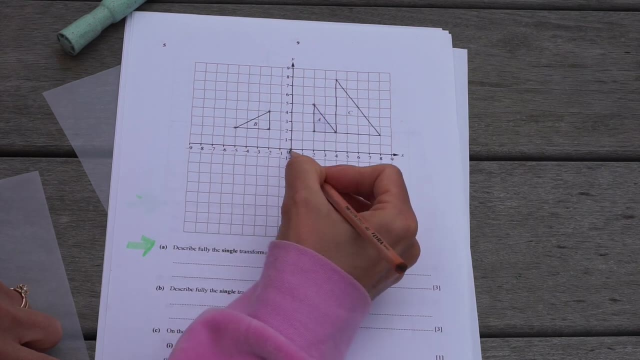 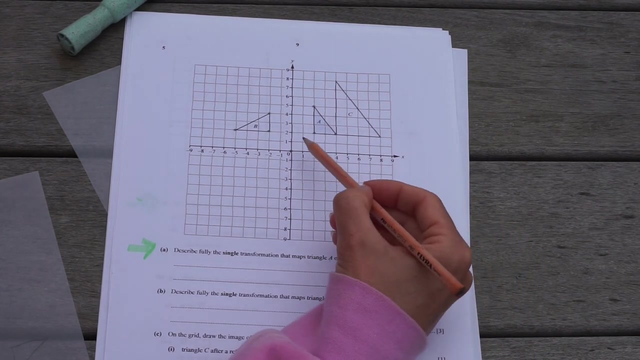 And lastly, the top of triangle A after the rotation changes to here, And those distances are also the same to the origin. Remember I said earlier in the lesson, The center of the rotation is equidistant. It's the same distance to all the different pairs of corresponding points in the two different shapes.